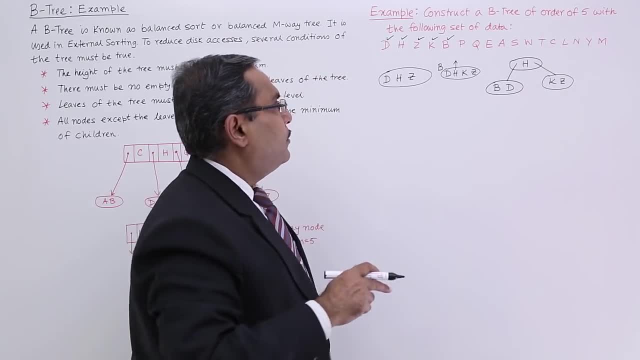 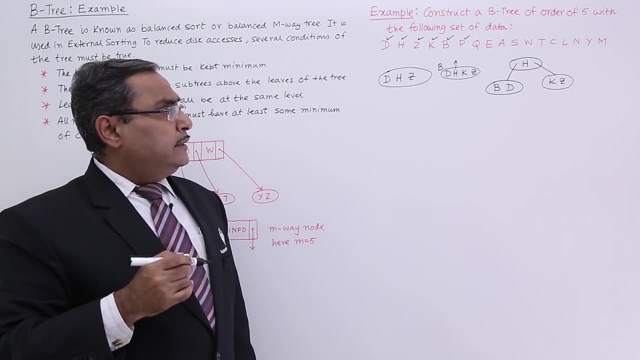 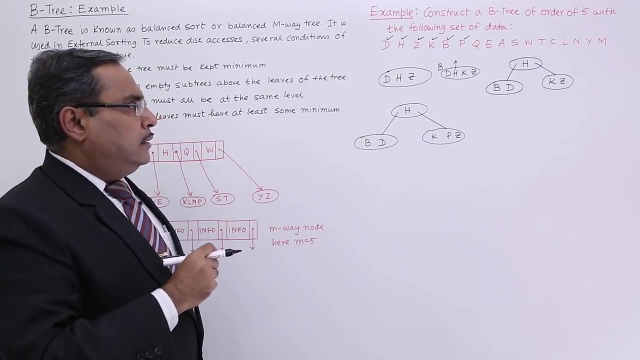 will be this. So they are coming in this way. Now P will be coming, So P is greater than H and P will be in between K and Z. So it will be coming like this. Now we shall be having Q. 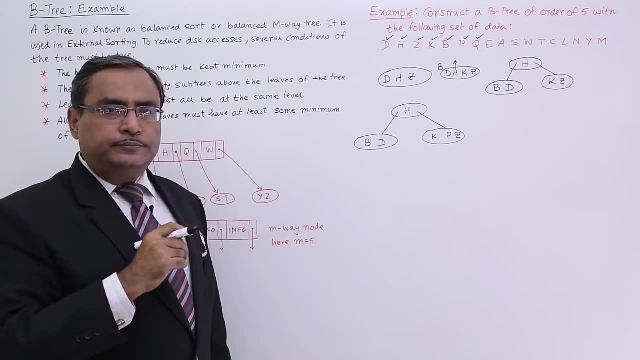 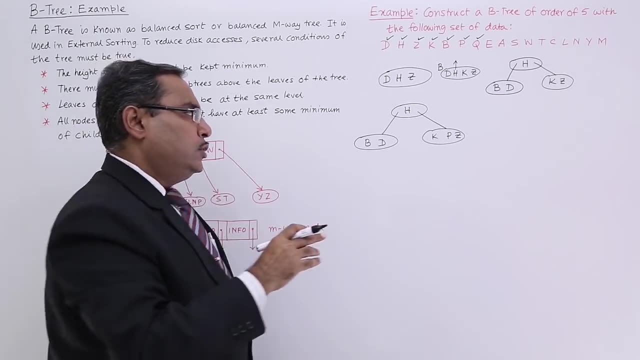 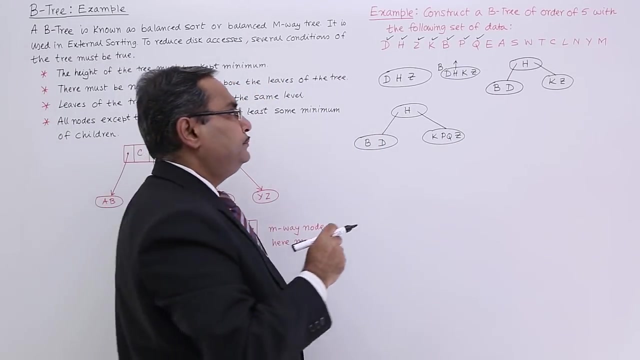 Q is greater than H, So Q will be getting inserted here. So Q is in between P and Z, So P will be coming here and Q will get inserted like this. So now E- E is lesser than H, So it will come to this particular node. 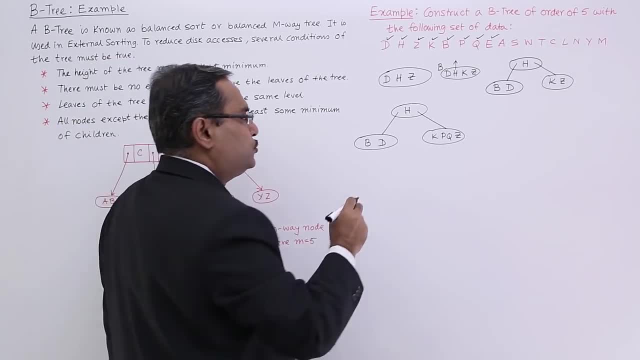 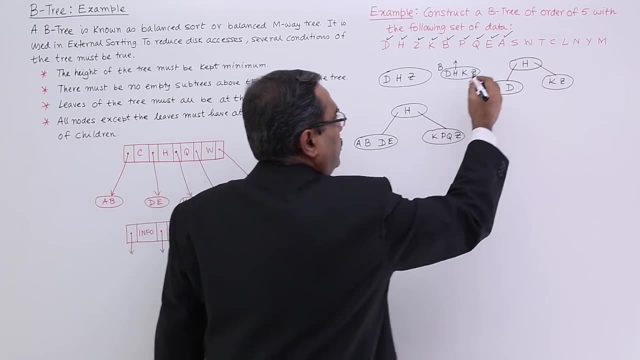 and E is greater than D, So E will be inserted here Next. A: A will be coming down here. A will be inserted here Next S- S is greater than H, So S will be going there. So now S will be in between Q and Z, So S will be here in between Q and Z. So the median is Q, So Q will go up and it will contribute with H. So it will be coming like this: Now W. 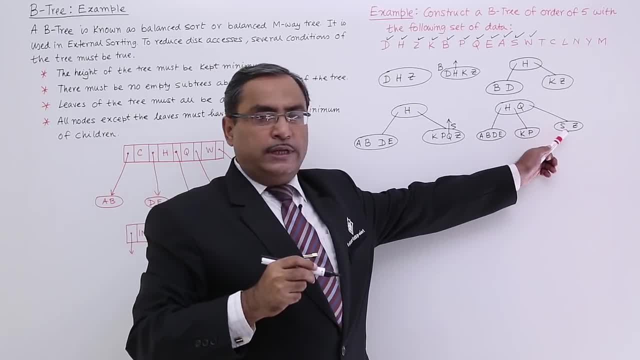 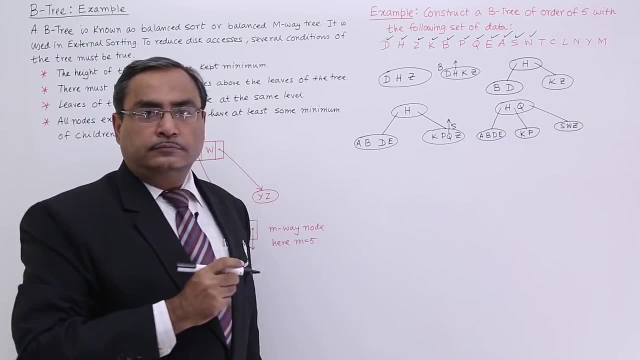 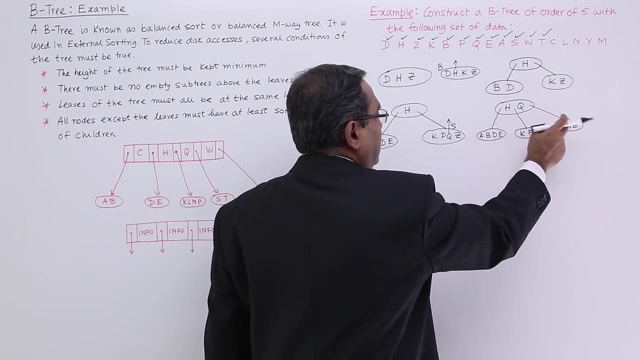 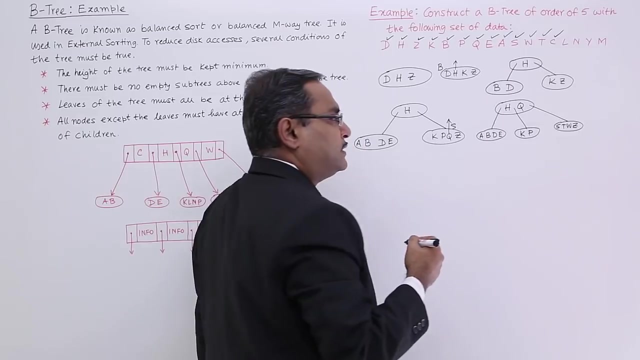 So W is greater than Q. So it will be going to this: Now W will be after S. Now we shall go for T, So T is greater than Q, and T will be just after S. Now we shall go for C, So C will be coming down here. Always remember the alphabetical order. 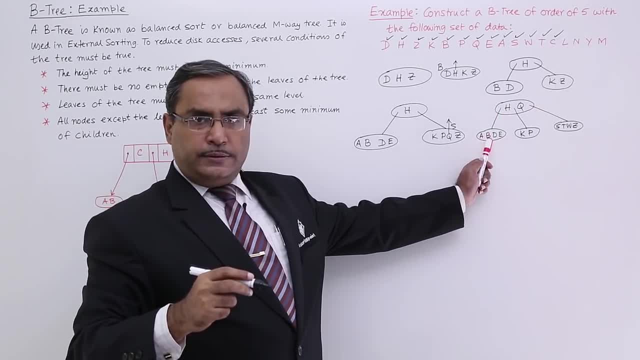 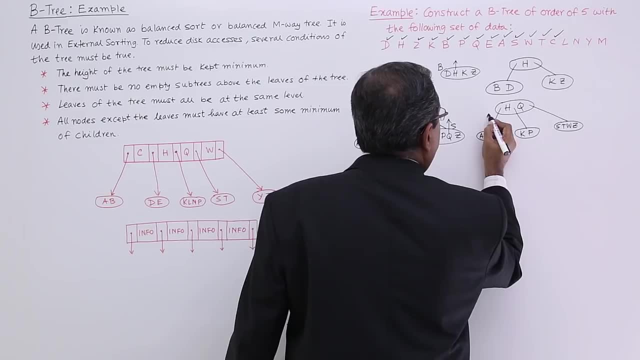 So C is lesser than H, So C will be coming down here, So C will be here and if you consider the median, C will be the median, So C will be going to this root node. So the tree will. 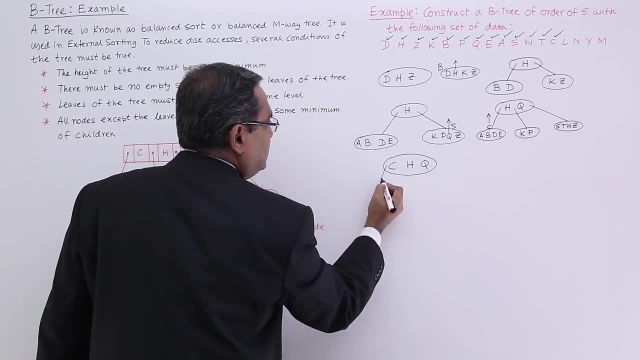 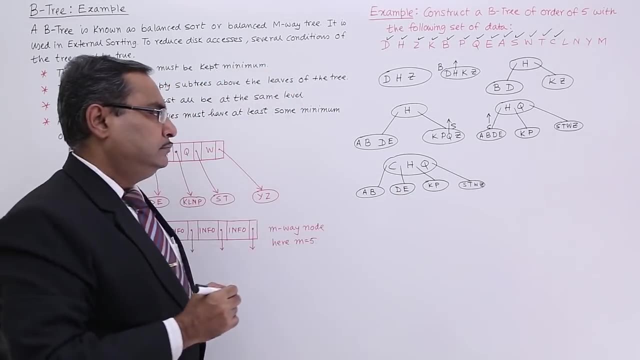 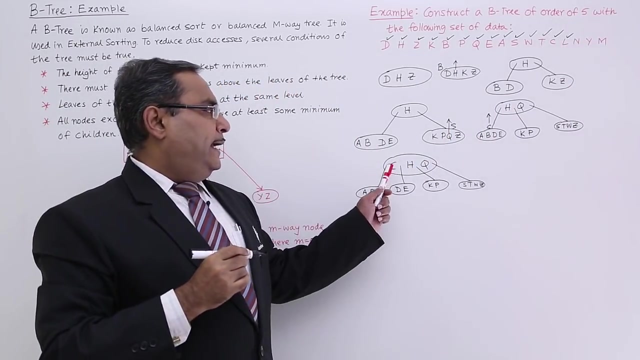 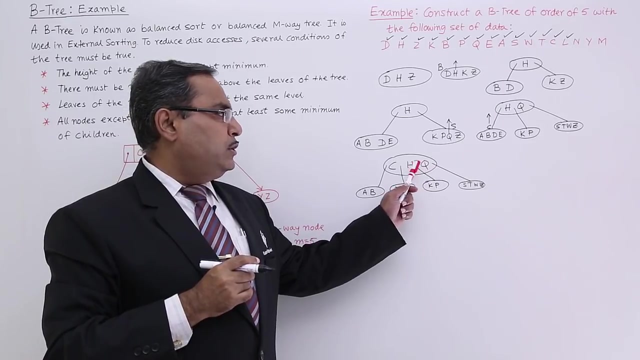 become lesser than C, greater than C but lesser than H up to this. So now we are going for L, So L is greater than C, L is greater than H, but L is lesser than Q, So it will be in between. 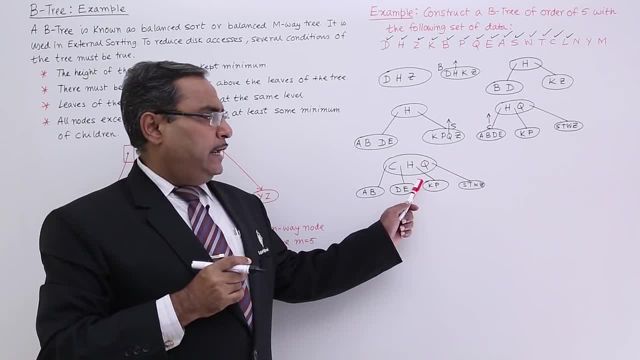 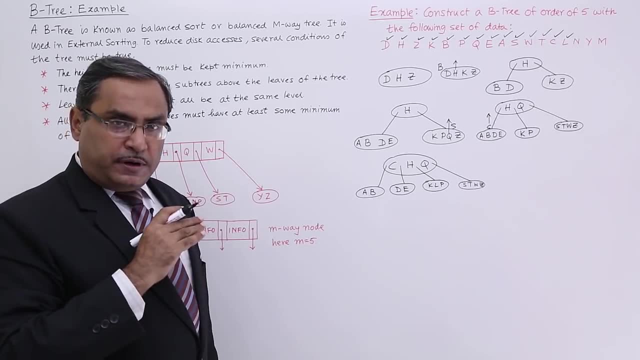 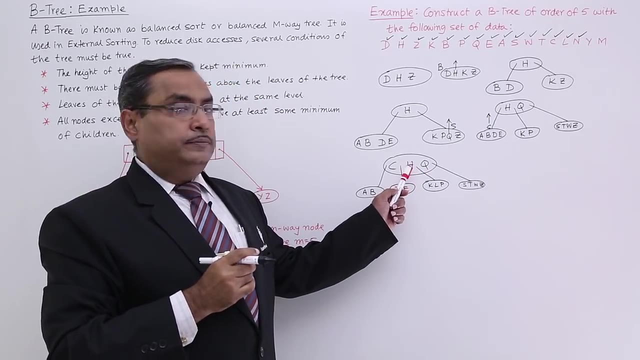 coming down here. L will be after K before P, After K before P. Now we shall go for N, Okay now. So now N N will be coming down here, So N will be coming down here, So N will be. 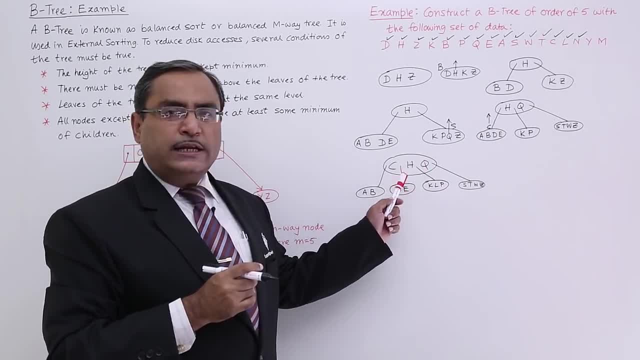 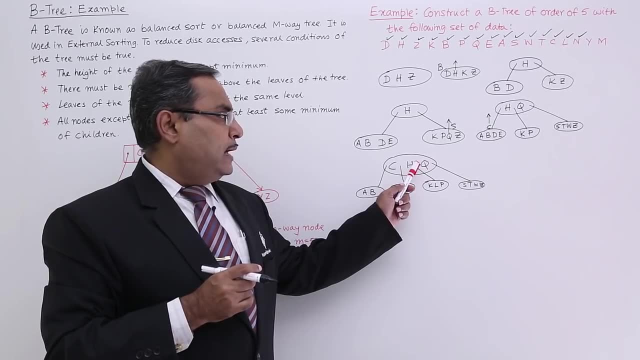 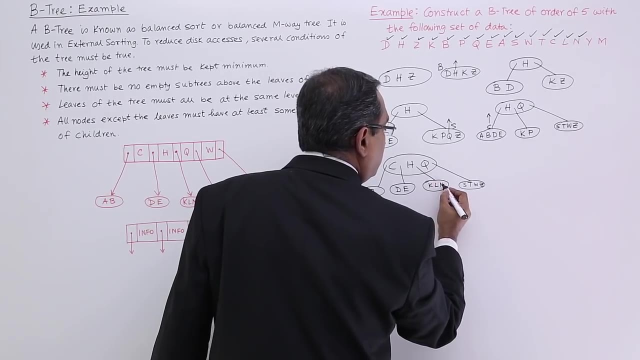 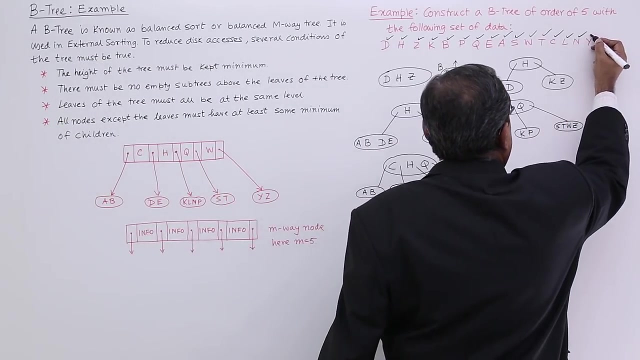 coming down. N will be before Q, because it is in between H and Q, So greater than C, greater than H, but lesser than Q. So N will be coming before Q. So it will be before P and after L, So N has got inserted, Next Y, So Y will be coming down here, So the 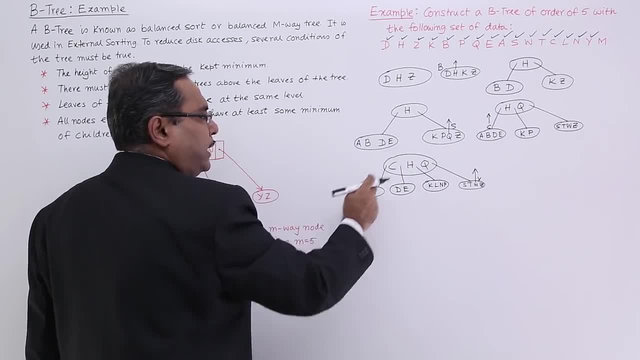 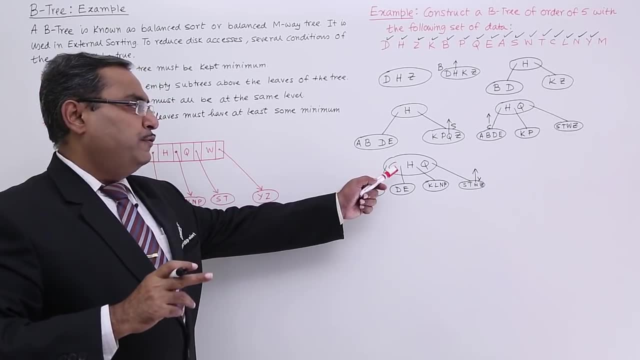 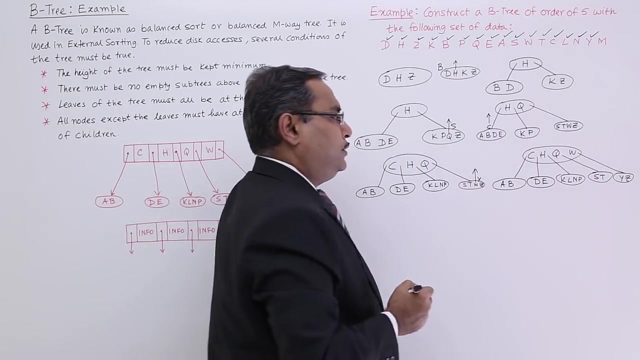 W will be contributing towards this root. Root can hold maximum 4 info, because 5 way, That means 5 links, That means 4 info. 3 info is there, So W can be accommodated here. So it will take a. 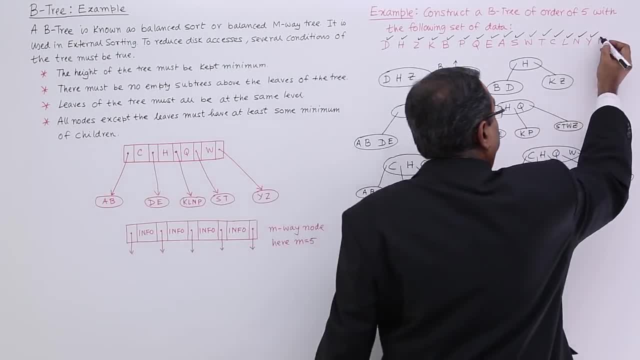 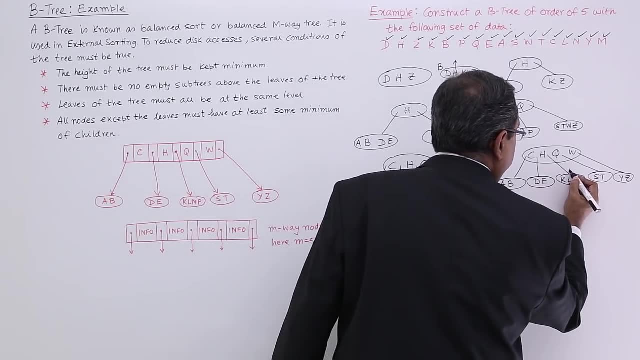 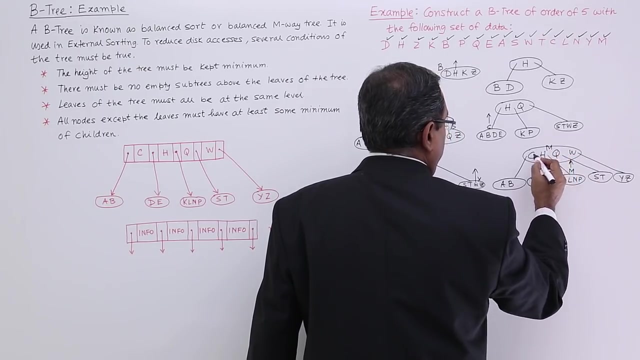 shape like this. Last one is M, So M will be coming down here, So M will be inserted in between L and M N. Middle most value is M, So M will go up, So M will come down here. but that is no space Already. 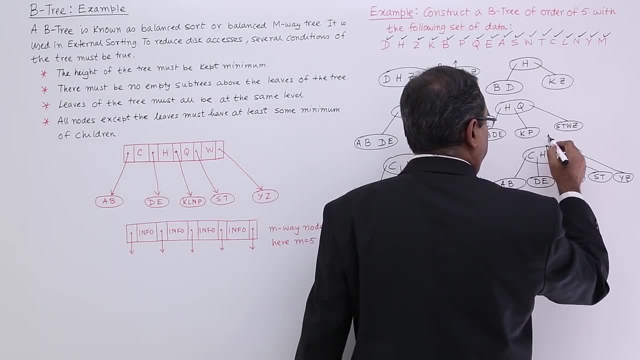 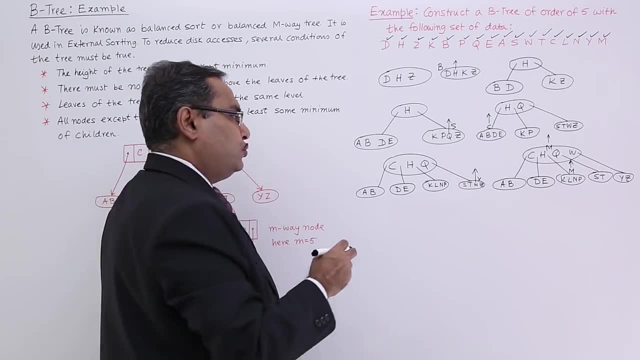 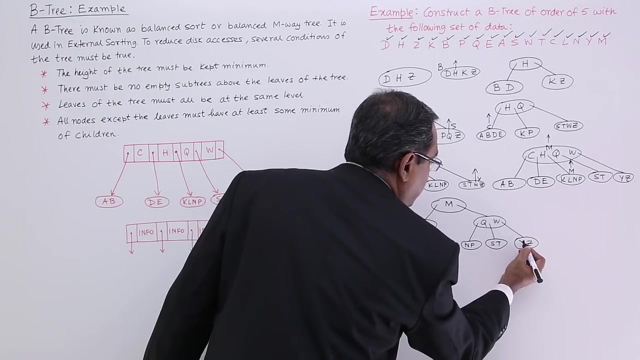 4. info are there. So M will be go up, So another level will get increased, Another height will get increased, So ultimately the tree will take the shape like this. So in this way the tree has been drawn ultimately. So that is the final tree. 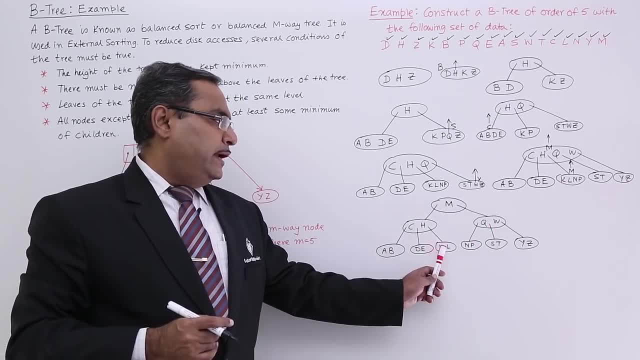 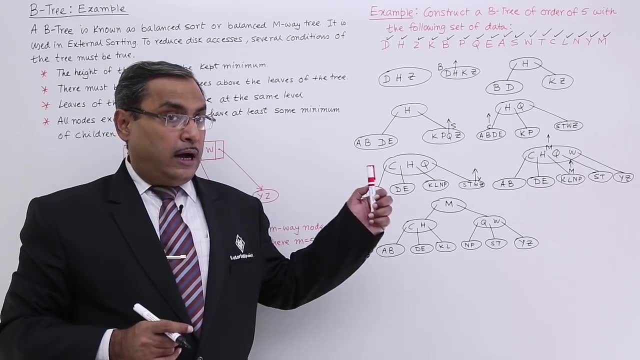 M, C, H, Q, W, A, B, D, E, K, L, N, P, S, T and Y Z. So in this way the B tree will get generated. So I have maintained all the properties, whatever we discussed in the earlier video, We 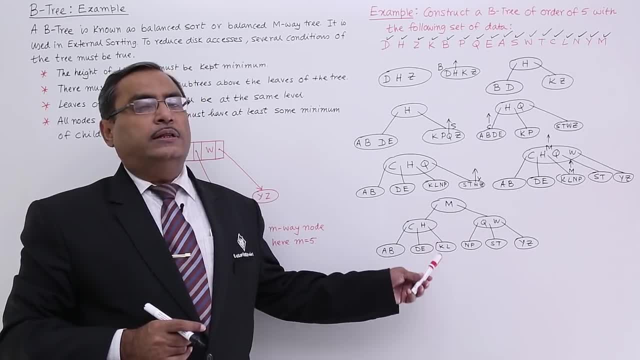 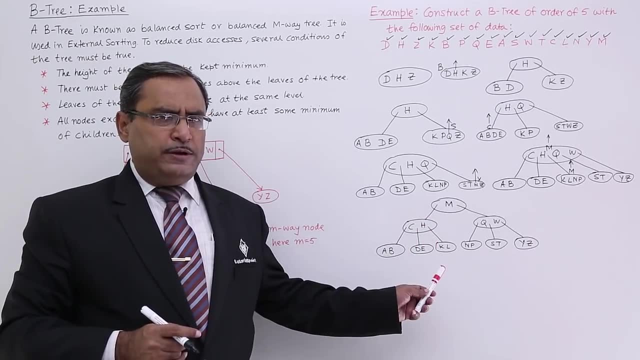 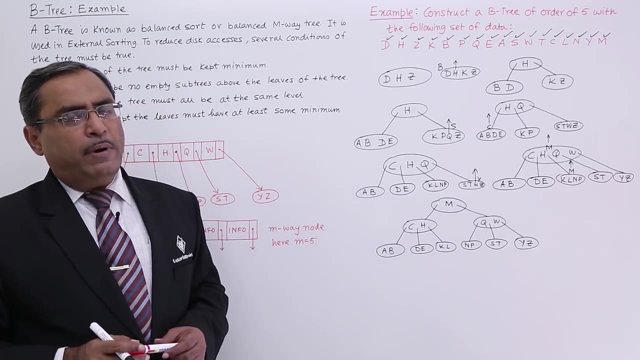 did increase the level of this particular B tree, the height of the particular B tree, as minimum as possible And for M O A B tree, or of the order of M B tree, we will be having M minus 1 number of link fields and we will be having M minus 1 number of info field, And that is why. 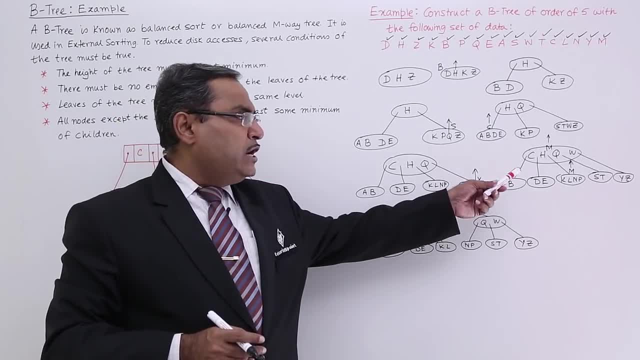 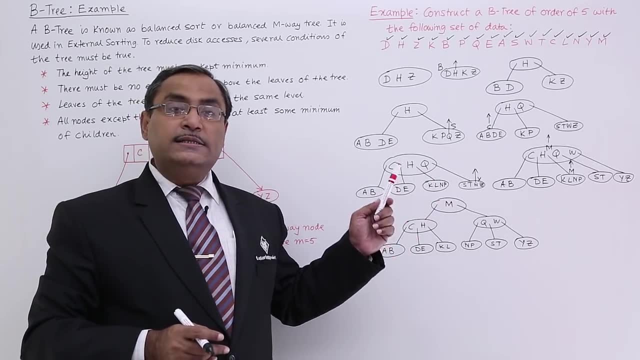 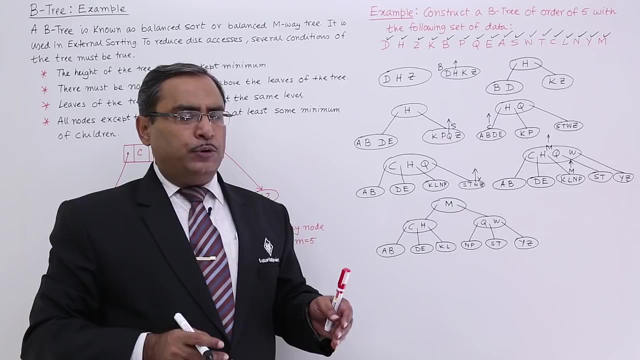 you see, here the value of M is equal to 5. So you cannot find any node which is containing more than 4 info And in this way, whenever we are trying to put one data inserted onto a pre-filled, completely pre-filled node, then the node will be splitted depending upon the median and the node. 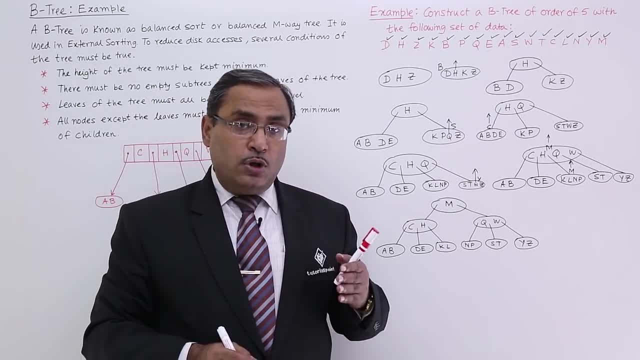 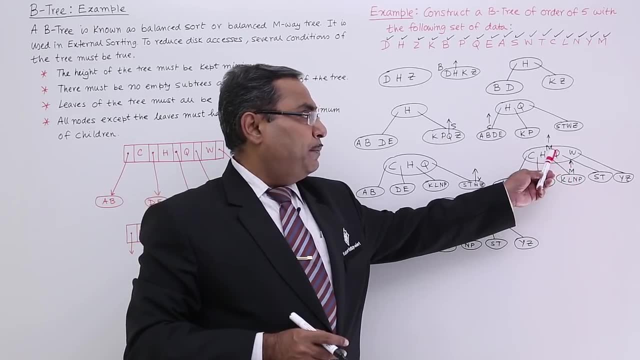 will be the respective info. the respective key value will be going to the parent node. If the parent node has got filled up, the node, the info will be going to the parent node. But if parent node has got filled up, then also another depth or height of the tree will get increased. 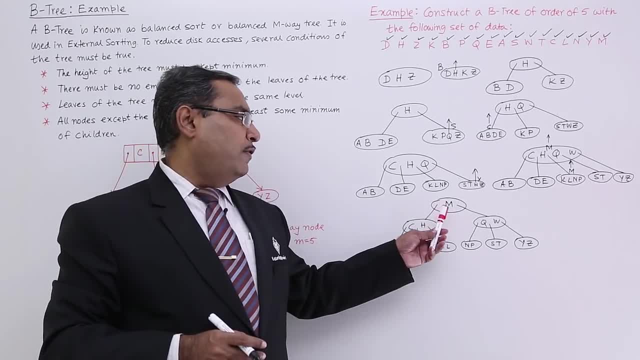 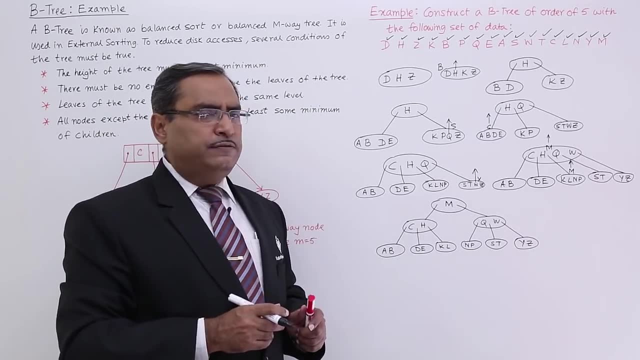 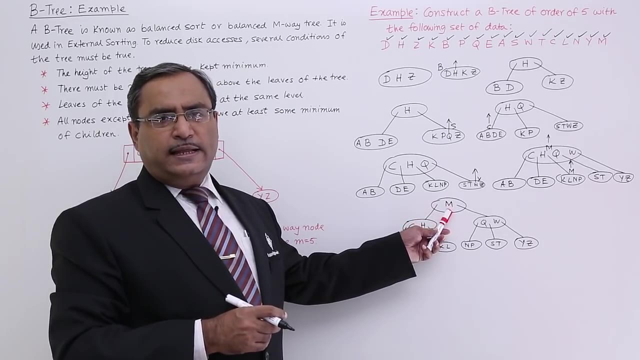 and another new parent will be formed, And in this way the children will be like this. So now let us go for searching. Do you want searching on it? Let us suppose I am searching for, say, F. I am searching for F, So now F is less than lesser than M, So I shall. 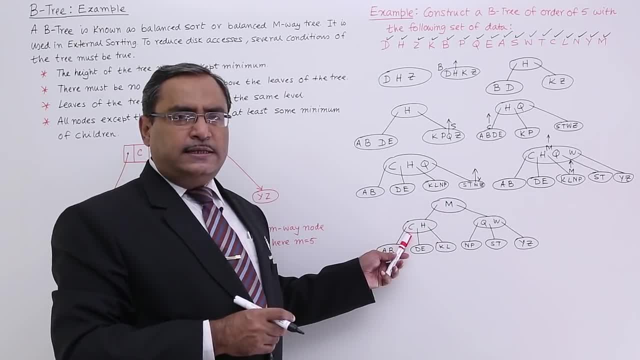 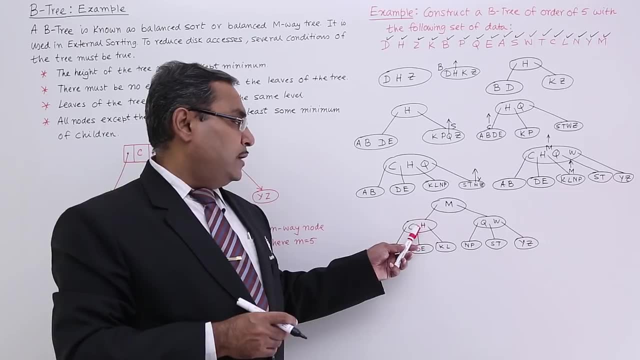 shall be coming down here. F is greater than C, So I will be going there Now. see, F is. F is lesser than H, So I will be coming down here. F is greater than D. F is greater than. 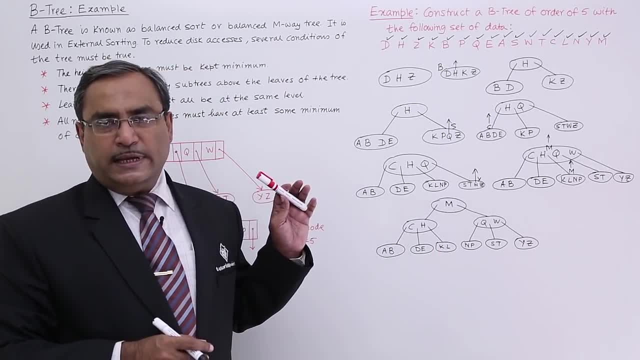 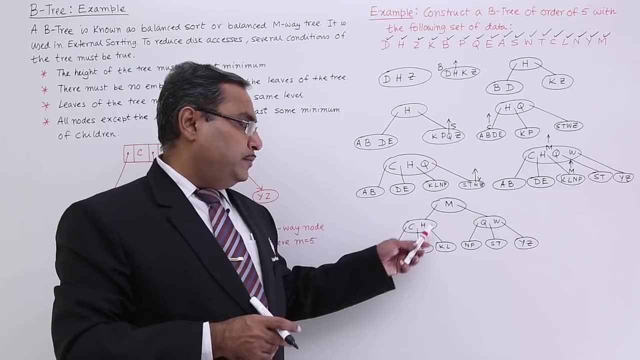 F But there is no F. So F is missing. So unsuccessful searching for a key value- F. In this way the searching will be done. You know, the height of the tree will be the decisive factor for the searching process. 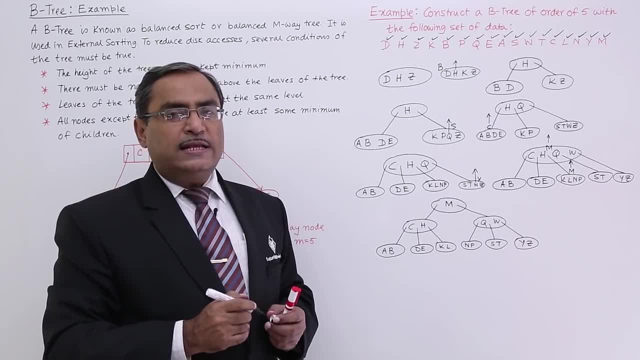 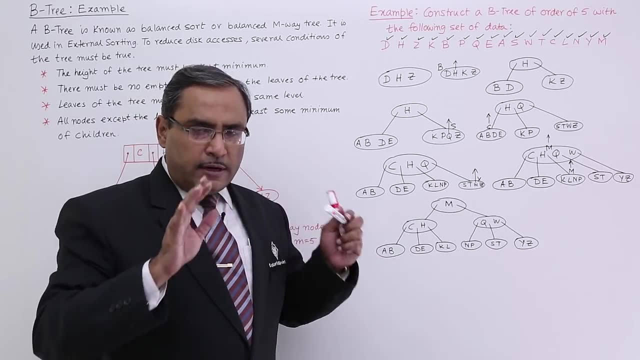 Complexity. So that is why we should express a B tree as minimum depth, as minimum height as possible. So I think previous video and this video has cleared up your doubts regarding this B tree. Thanks for watching this video. 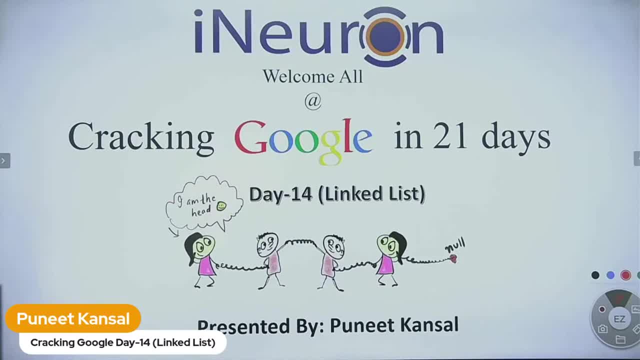 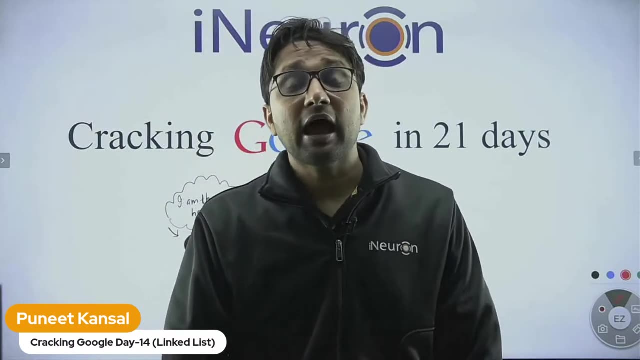 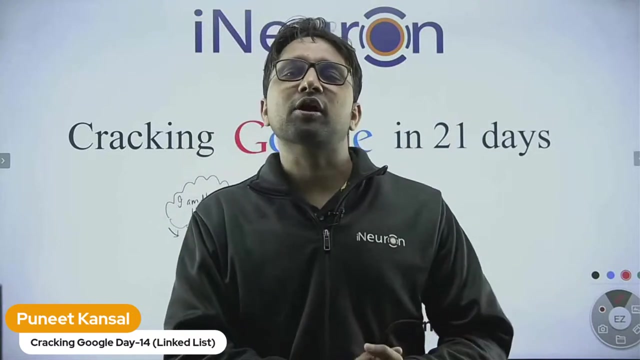 Hello everyone, welcome back to the series of tracking Google in 21 days. My name is Puneet Kansal. I'm the instructor for this particular series. If you are targeting for Google or any other product based company, this series will definitely help you. Why?